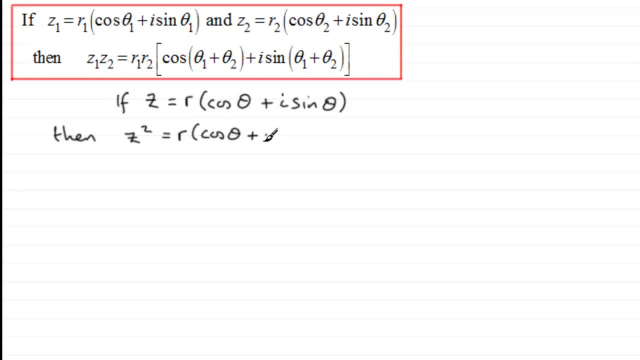 R cos theta plus i sine theta, and we would multiply that again with R cos theta plus i sine theta And by the result up here, then this must be equal to R times R R squared, and then all we need to do now is just add the arguments together. 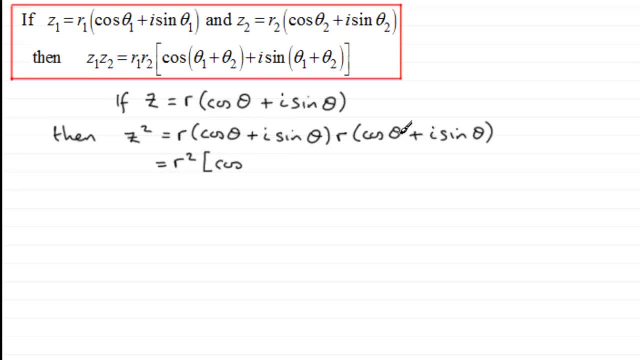 so we get the cos of theta plus theta, cos of 2 theta, and when it comes to the sine, it's going to be I sine 2 theta. now what happens if we extend it again and we look at Z cubed? okay, if we were to look at Z cubed, think of this then, as Z 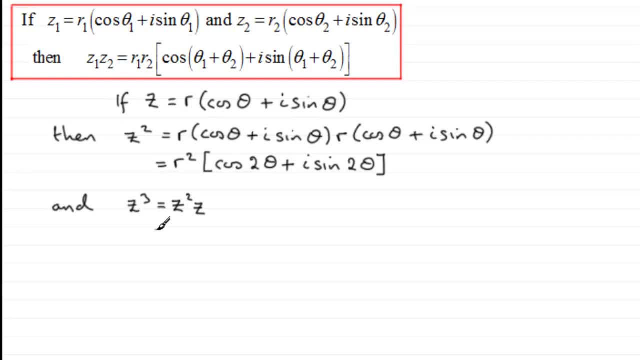 squared times Z. well, we've already got Z squared. Z squared was R squared multiplied by cos 2 theta plus I sine 2 theta. and if we multiply this result with Z- Z being our cos theta plus I sine theta, then what are we going to get? well, 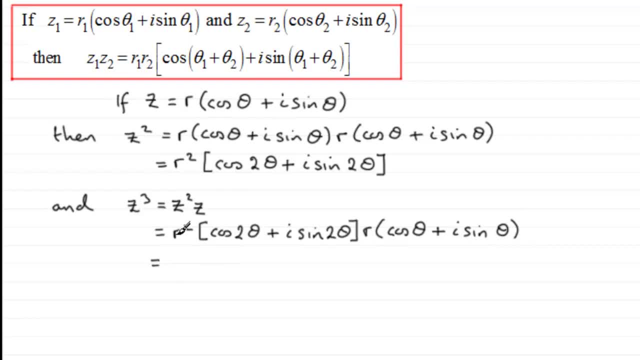 by the rule of, well, by the rule of, here again we've got R squared times R, that's going to be R cubed, and then we just simply add the two arguments together, so we get the cosine of 2 theta plus theta, in other words 3 theta and the same with the sine we've got I. 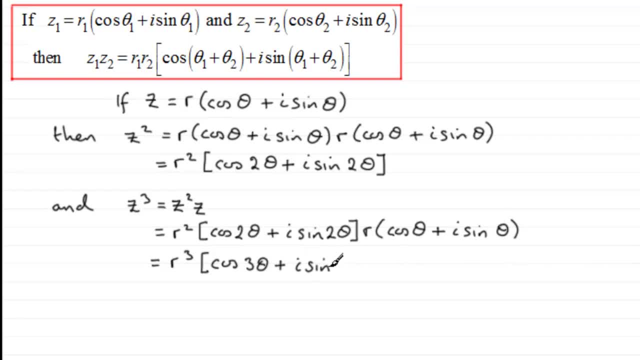 sine of 2 theta plus theta, which is 3 theta. now, if we were to work out Z to the power 4, it would be Z cubed times another Z, and by following a similar pattern to this, it turns out that Z to the power 4 is equal.